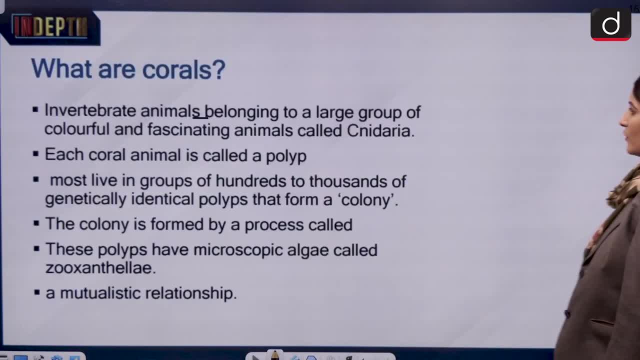 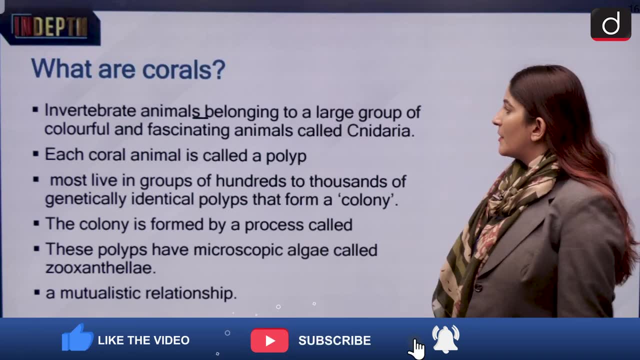 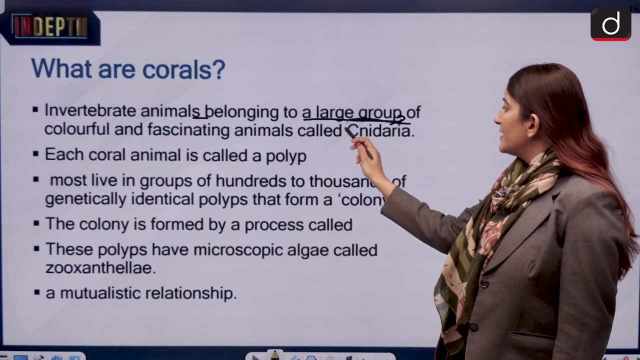 as well as the conclusion. These many topics are going to be discussed. Let us start with corals. What are corals? These are invertebrate animals, Remember them. They belong to a large group of colourful and fascinating animals and it is known as Tenderia. Each coral animal is 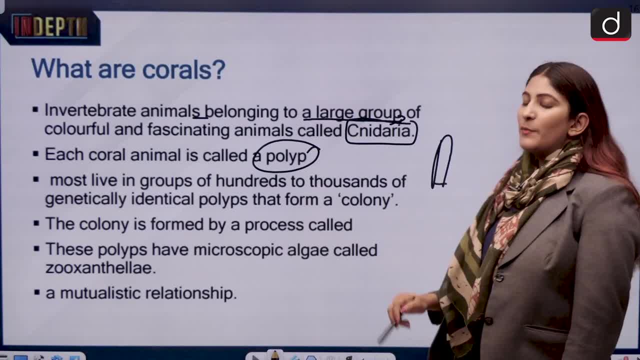 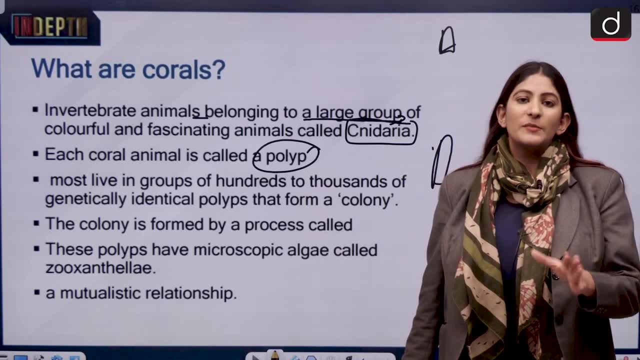 known as a polyp. This is a polyp, supposedly, and these polyps do not live individually. That one polyp is here. another polyp is there, No, as we know, to produce corals. corals are not protected. Any species wants to live in colony, So they live in colonies and the colony formation. 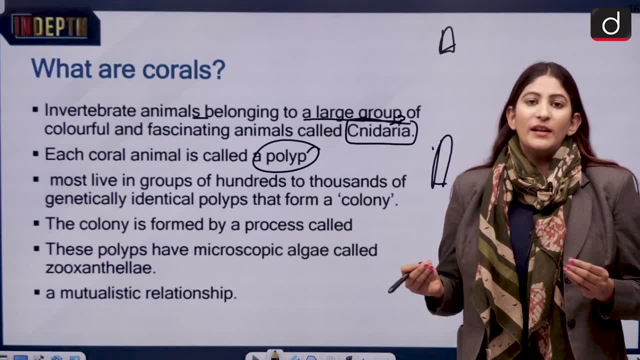 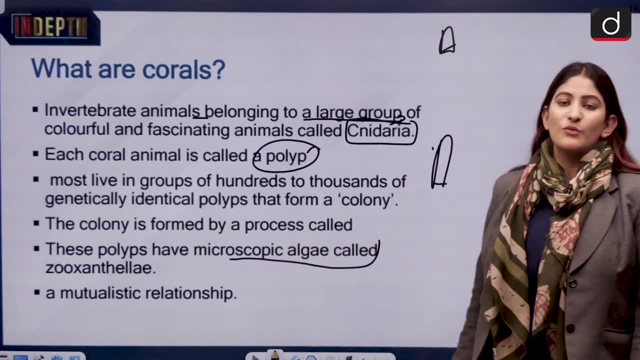 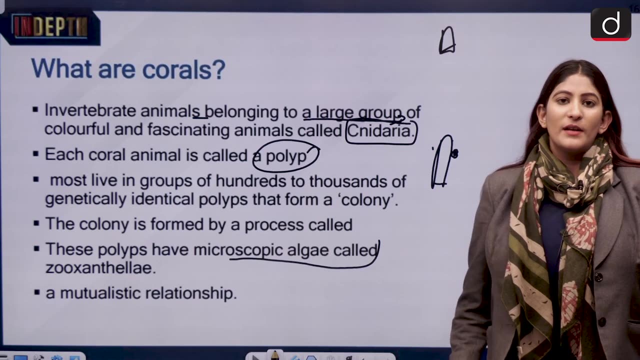 is known as budding, And they bud along. that is why they form a colony. Now, these polyps, they have microscopic algae which is known as zooxanthellae, So these polyps have zooxanthellae in them. Now, zooxanthellae and the coral polyp, they have a unique relationship and it is known. 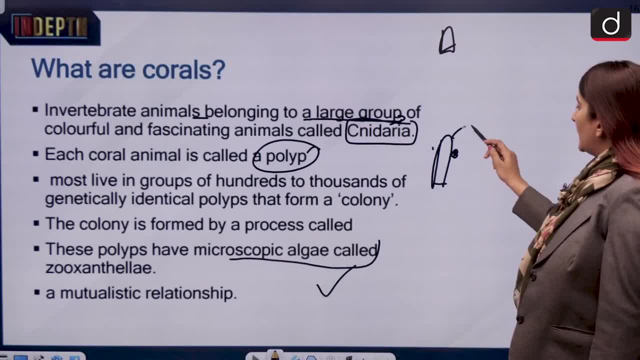 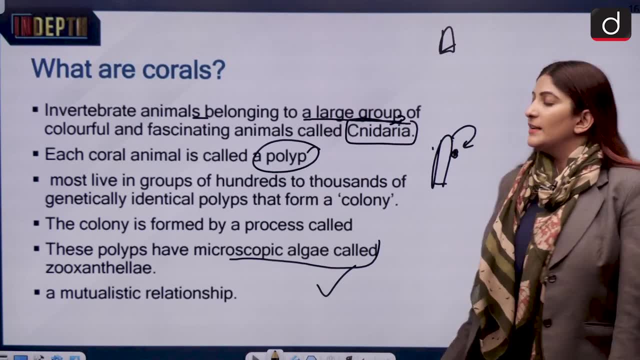 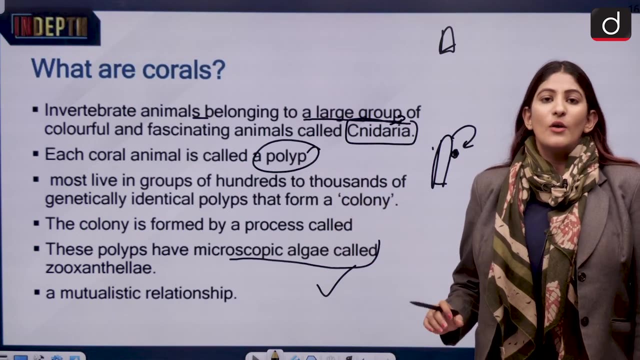 as a mutualistic relationship. The polyps help the zooxanthellae to get stuff for photosynthesis, and in return the zooxanthellae provide them such material so that they can carbonate their calcium. Okay, so first we can. 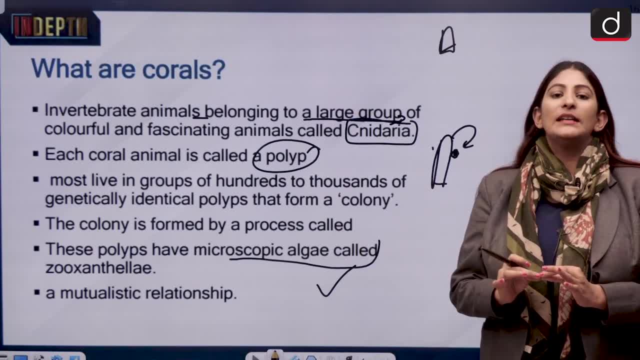 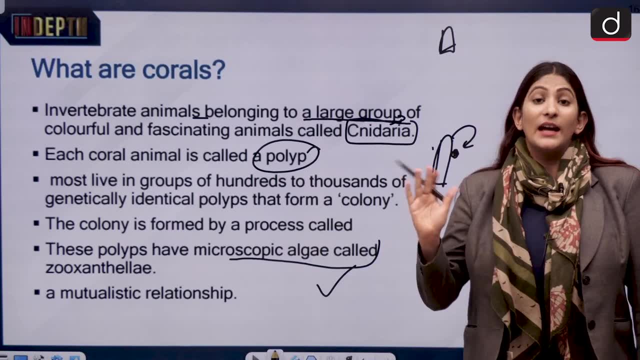 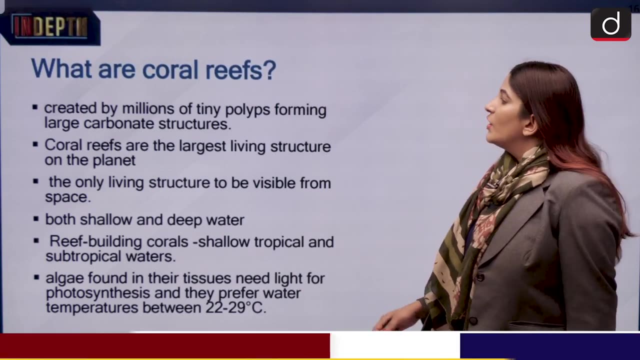 say what is a mutualistic relationship? That both the organisms are helping each other in some manner. and because of zooxanthellae, only the colourful nature of the polyps can be seen. Now coral reefs. of course we know corals, now Coral reefs are created by millions. 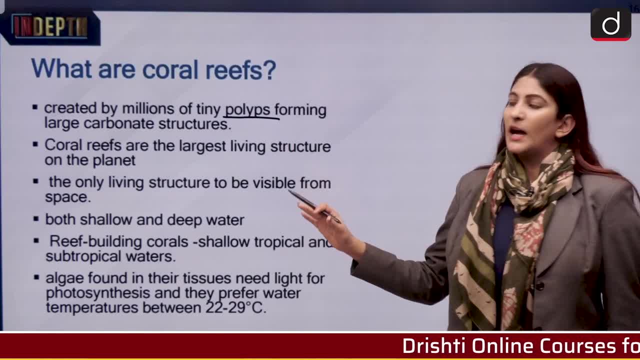 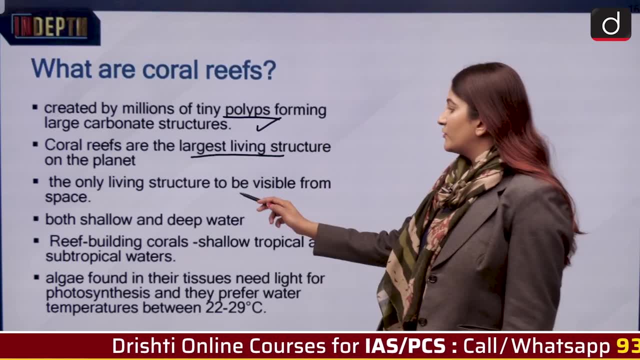 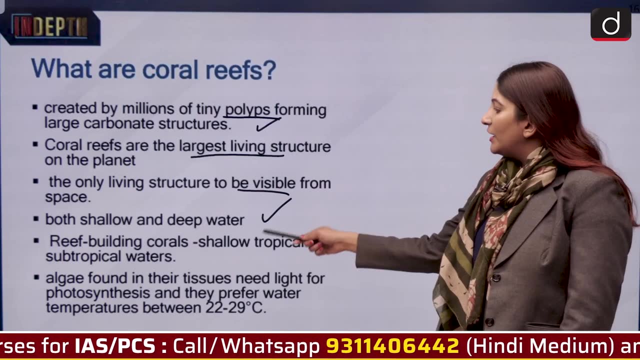 of tiny polyps which form a non-carbonate structure. Coral reefs are the largest living structure on the planet and, interestingly, the only living structure that can be seen from the space. They live in both shallow, less water and deep water. Reef building corals. 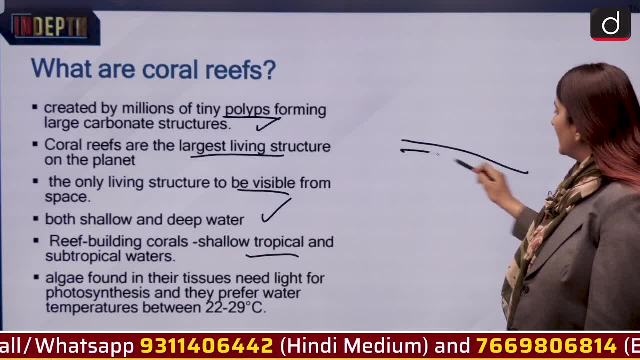 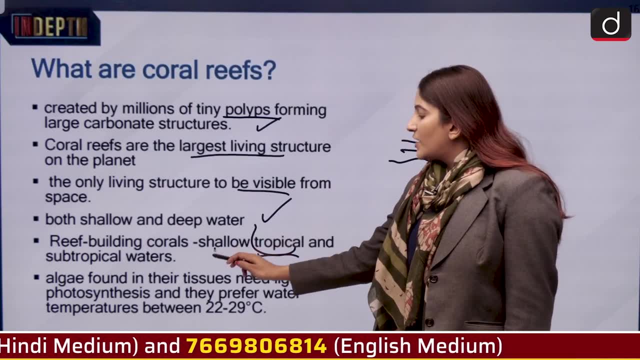 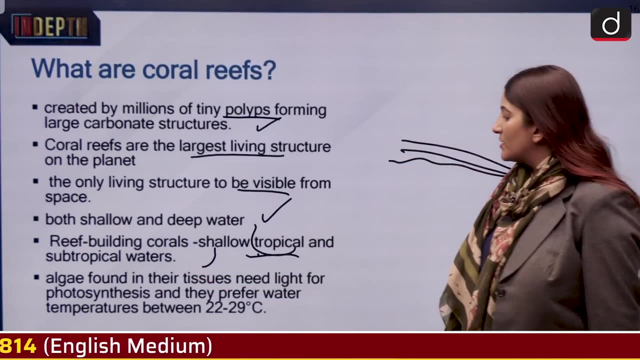 although if we talk about corals that build reef, that means along shorelines of the continents. they can be found only in tropical, shallow tropical and shallow subtropical waters. Okay, because the algae, which is important, zooxanthellae, which is important to. 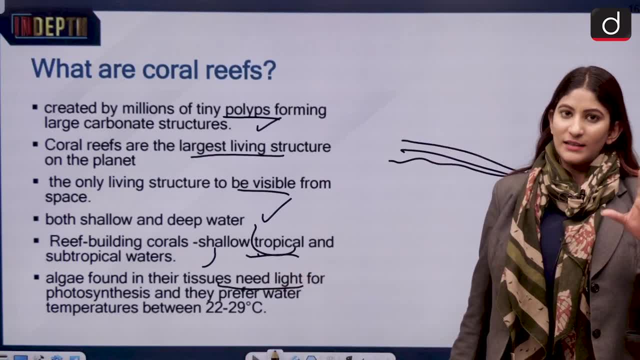 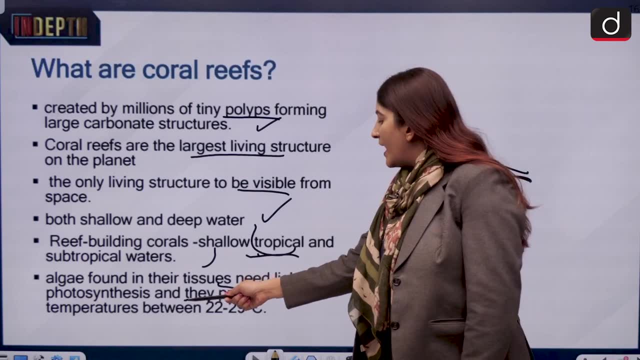 live in the tissues, they need light for photosynthesis and here in this region, in designated latitudes only, we can find the reef building corals because of that, and they prefer water temperatures between 22 to 29 degree Celsius. Moving on, 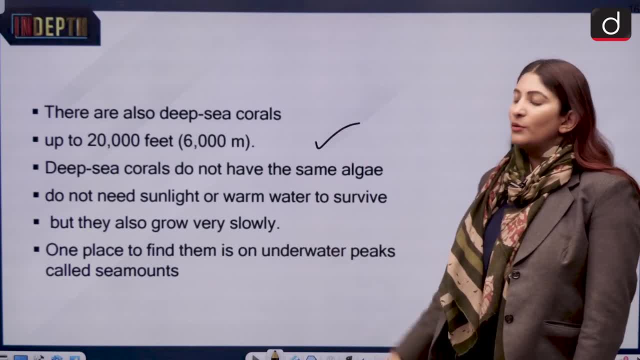 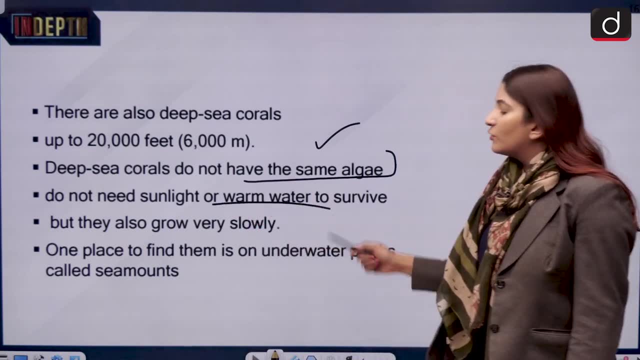 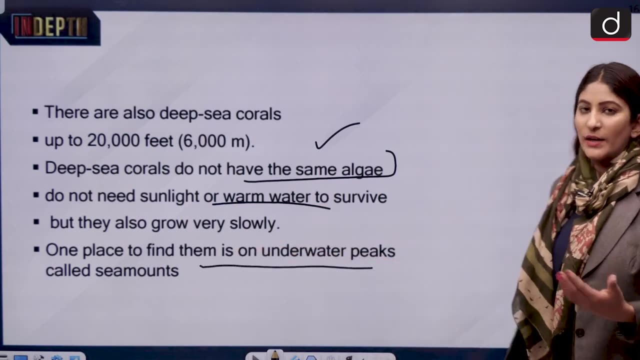 there are also deep sea corals, and they can be there up to 20,000 feet. They do not have the same algae like the shallow ones have. They do not need sunlight or warm water to survive. that is why they grow slow. One place to find them is on underwater peaks, which are called as sea mounds. Okay, now, three types of 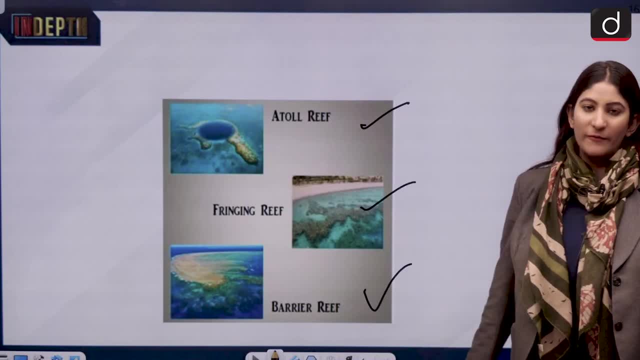 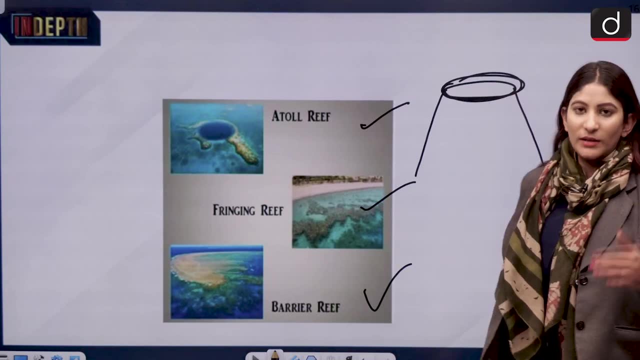 reefs are there: atoll reef, fringing reef and barrier reef. Atoll reef can be found on the mouth of the volcanoes, the, which were actually found duringbnאת. the했Reafs are found like that сол above water for a period of time when they submerged at the mouth of the. 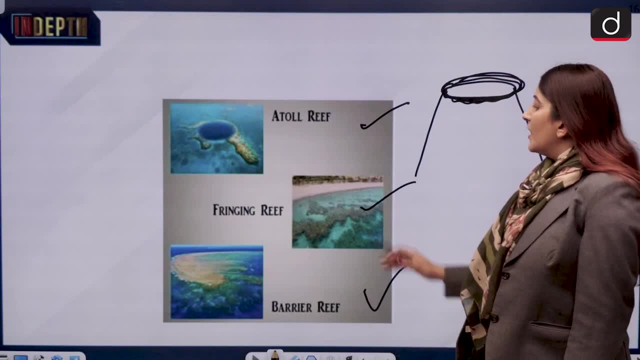 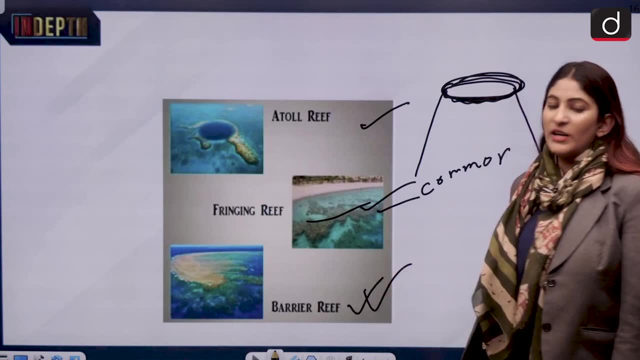 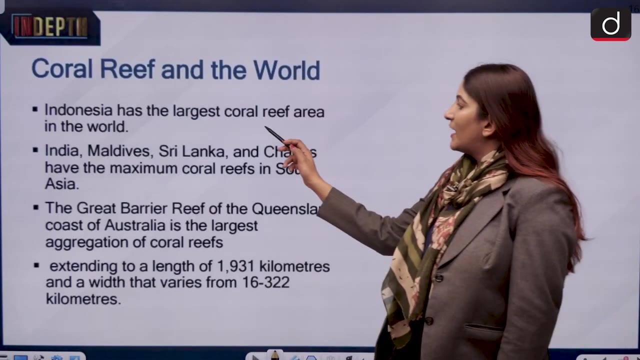 volcano, the atoll started building itself. then fringing reef- this is the most common reef- okay, most common one is fringing- and then we have barrier reef which forms on the shoreline, such as the Great Barrier Reef of Australia. now Indonesia has the largest coral reef area in the world: India, Maldives, Sri. 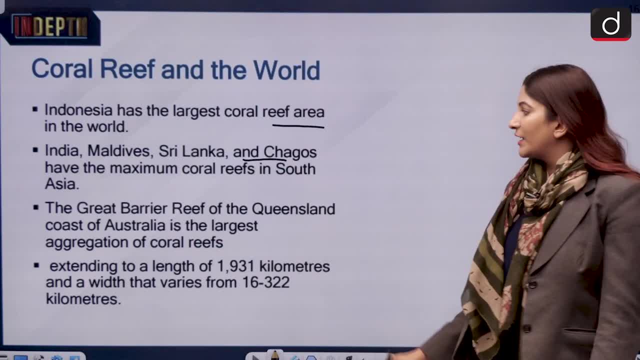 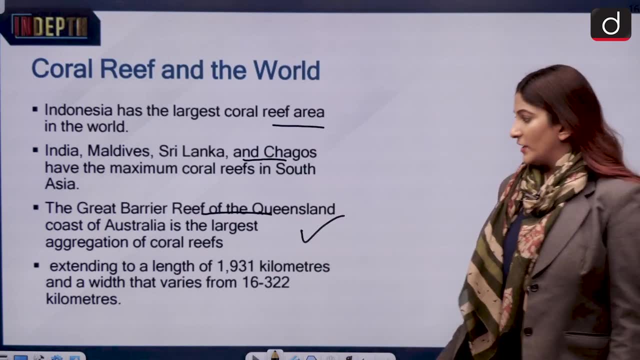 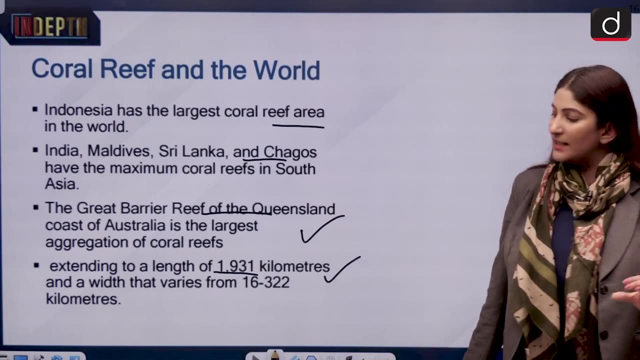 Lanka and Chagos. they have the maximum coral reef in South Asia. the Great Barrier Reef of the Queensland coast of Australia is the largest aggregation of coral reefs. they extend to a length of 1931 kilometers. they have a width that varies from 16 kilometers to 322 kilometers, and this is the most impacted. 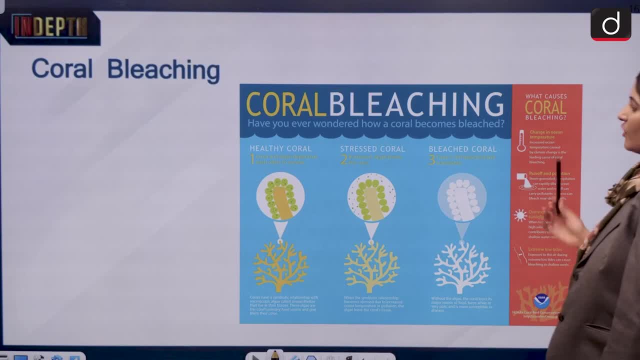 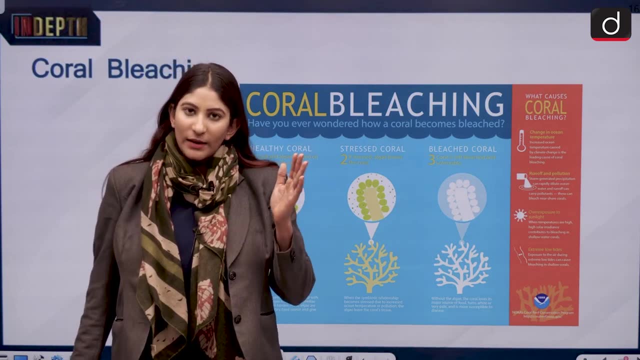 by coral bleaching. okay, moving on, let's talk about coral bleaching. see coral bleaching by the name. you can see in the description of this video. you can see it's. it's something like when the corals leave their color. okay, they do not have. 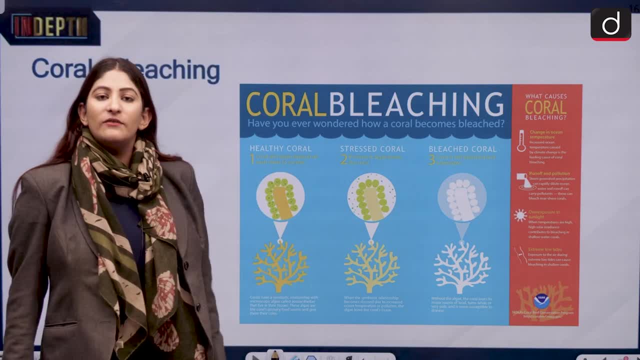 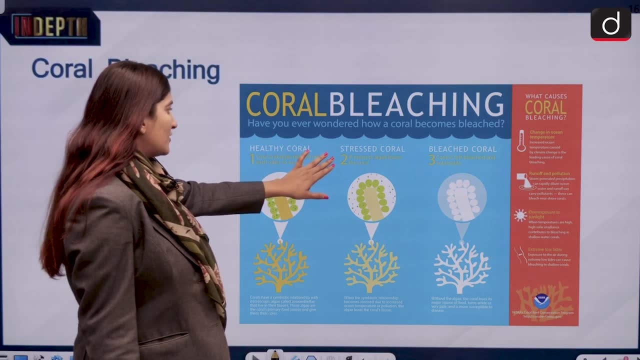 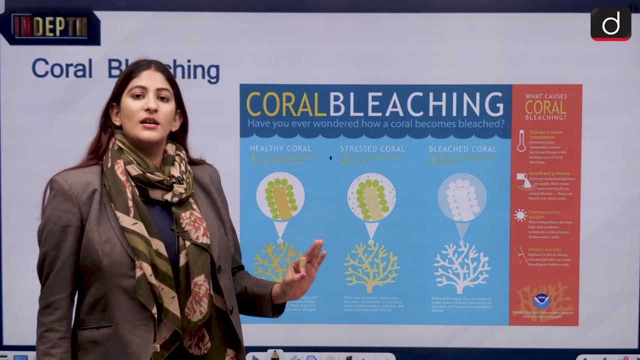 their color anymore. a healthy coral is a coral in which polyps are there and zooxanthellae. they are living happily together. okay, and they have, of course, the second part, that when any change in temperature of the water pollution occurs, degradation of water quality occurs, eutrophication occurs, in which 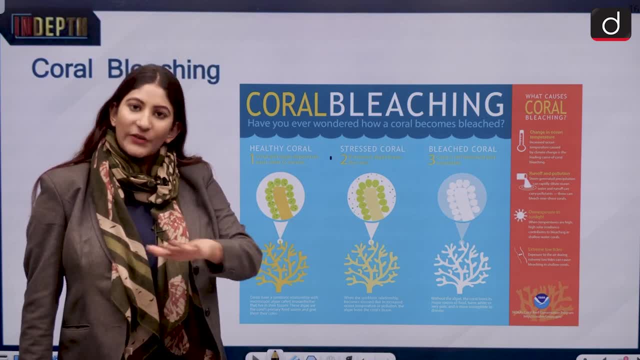 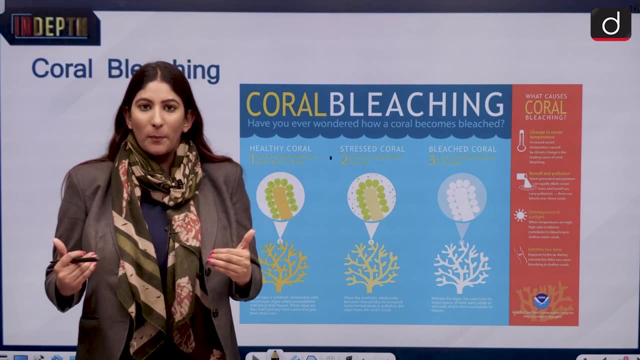 algae is another sort of algae is also a thrive in the water, so that sunlight cannot reach them. they become stressed, they are in tension that they are not getting the proper nutrients. so when that happens, these zooxanthellae starts leaving the corals. now, when zooxanthellae 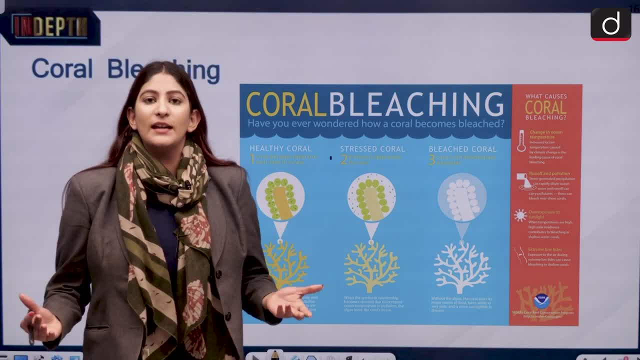 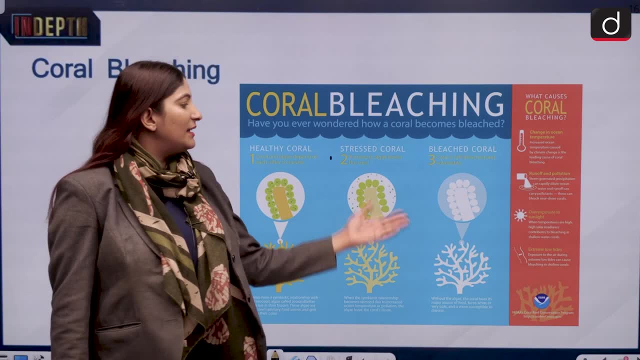 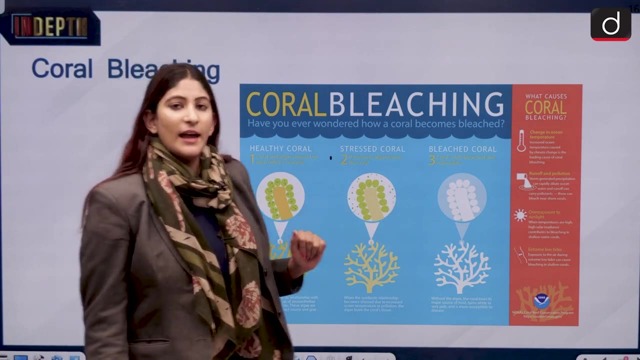 leaves the corals. what happens? the corals? they do not have anything to provide them the food and the color, and hence we see that coral bleaching is done and these can be maintained. they can be, you know, reclaimed as a healthy coral if we start taking care of them. so if we are talking about 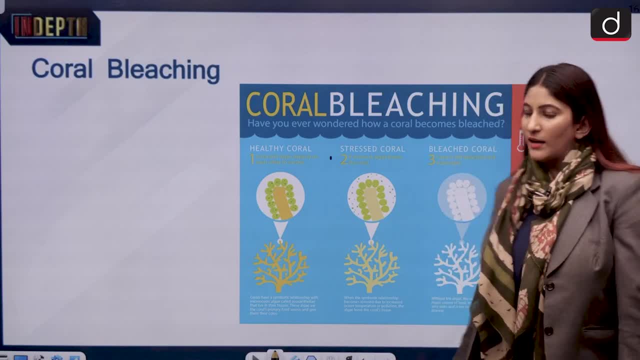 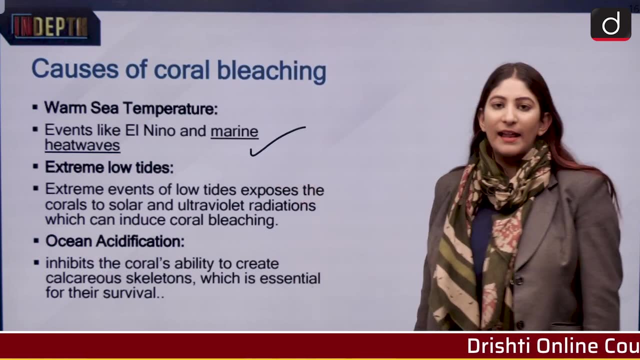 corals, we have to know about zooxanthellae. remember that zooxanthellae is our friend. now let's talk about causes of coral bleaching. when events such as El Nino and marine heat waves occur, there is a specific temperature in which the 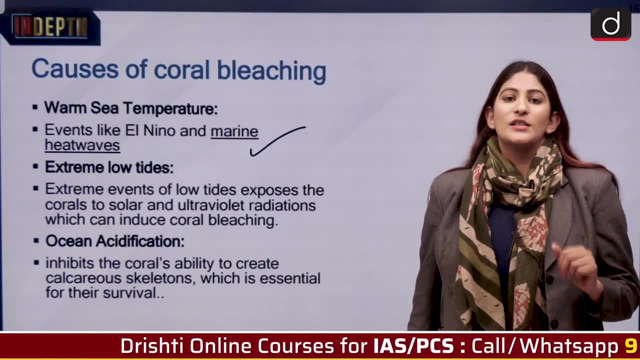 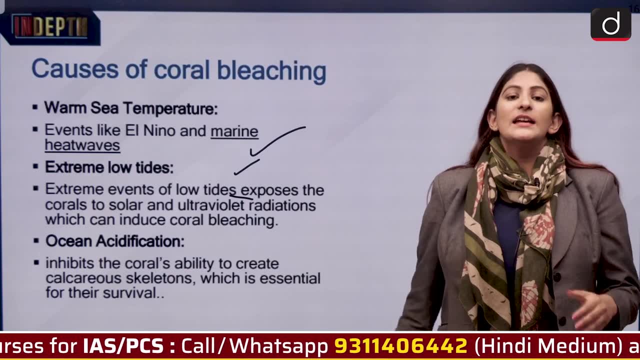 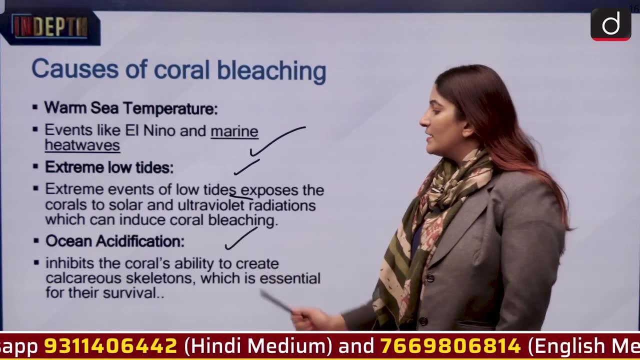 corals thrive. but if the temperatures change, the corals become stressed. zooxanthellae leaves them extreme low times. what happens when there are extreme low tides? these corals are exposed to too much sunlight and too much pollution. then also zooxanthellae says bye-bye to corals. then there is 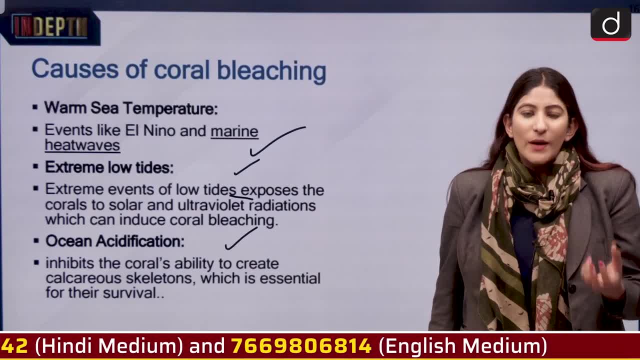 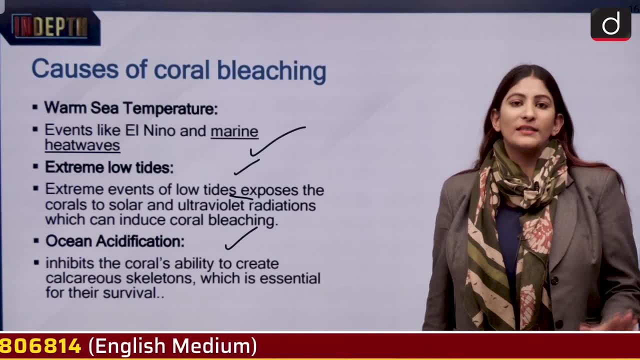 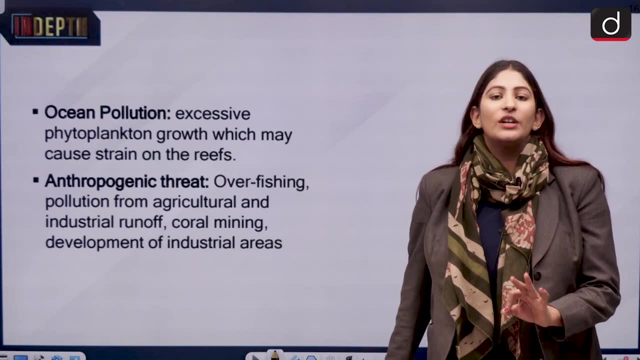 ocean acidification. as we know, oceans sequester carbon dioxide and because of that the acidic nature of the water increases. and when that happens, zooxanthellae again says bye-bye to the corals. now the next one is ocean pollution when too much nutrients go into the water in the form of fertilizer. 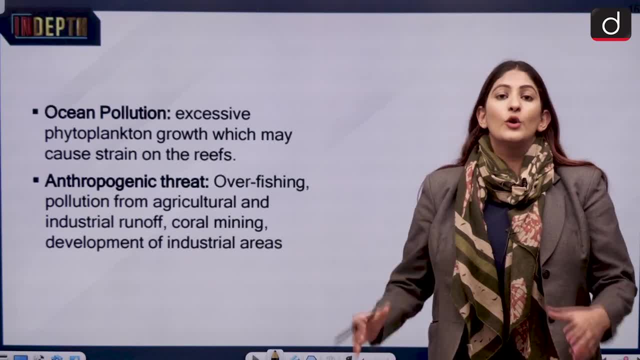 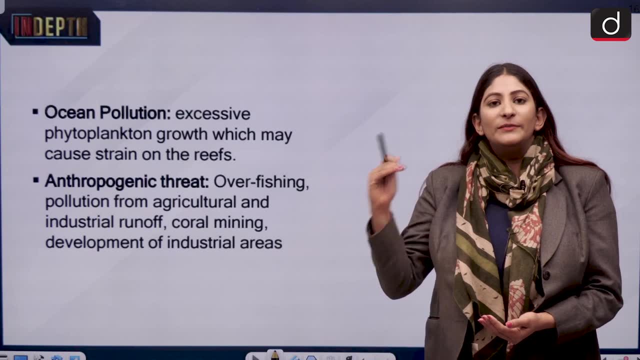 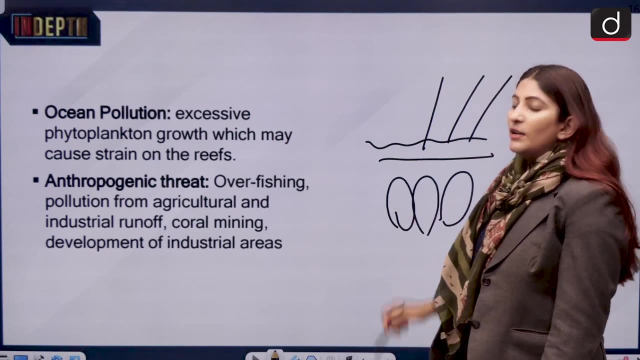 pesticides, then that can result in growth of phytoplankton. too much nutrition has gone and because of that phytoplankton start occurring. they, phytoplankton are here. they will block the sunlight and the poor corals polyps. they will not get the 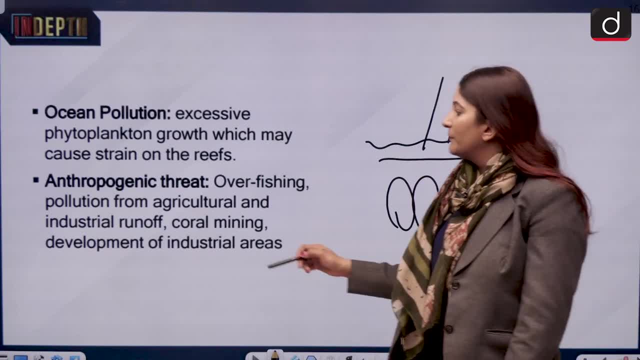 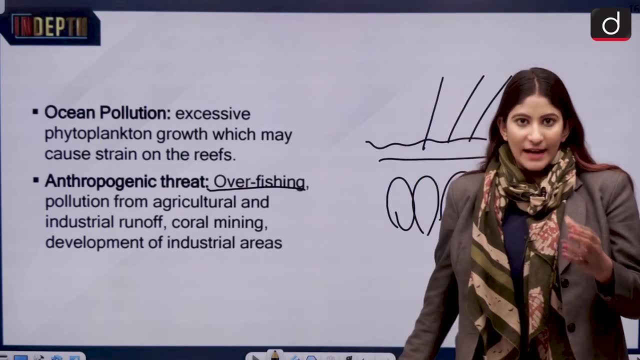 proper sunlight and then zooxanthellae again will leave them anthropogenic threat such as overfishing. fishes are also important to corals and in the net of the fishing corals get superfluous sunlight, so these corals will be able to survive the 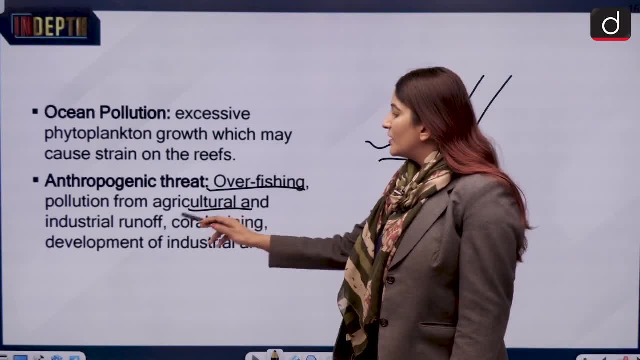 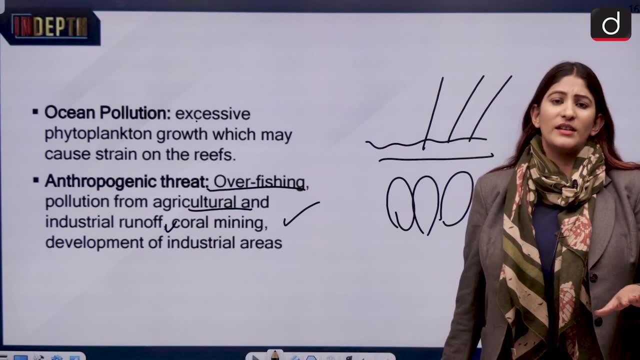 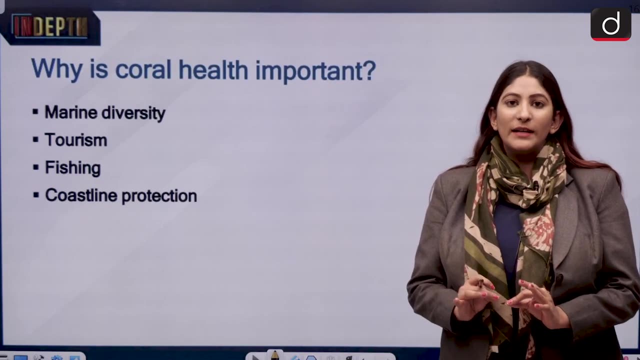 stuck. That is also another problem: Pollution from agriculture and industrial runoff, which leads to ocean pollution. Coral mining and development of industrial area around the coral areas is also a threat. Now, if we talk about why is coral health important In order to maintain? 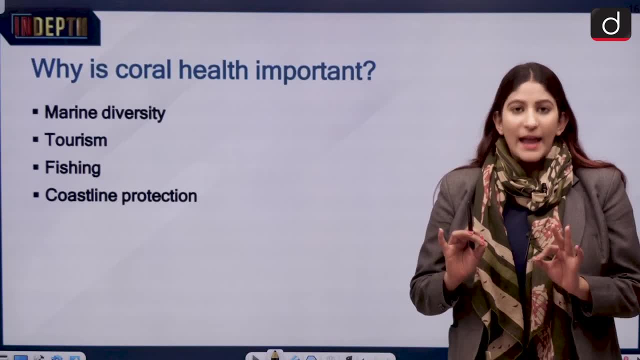 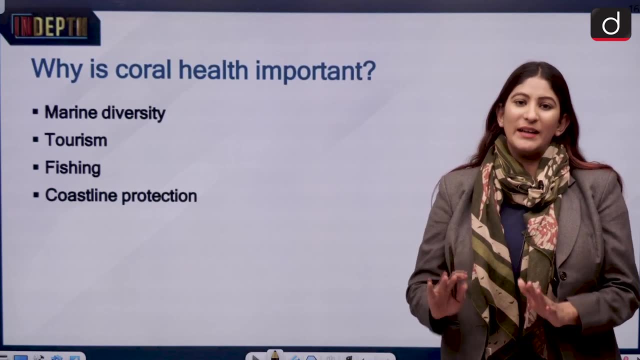 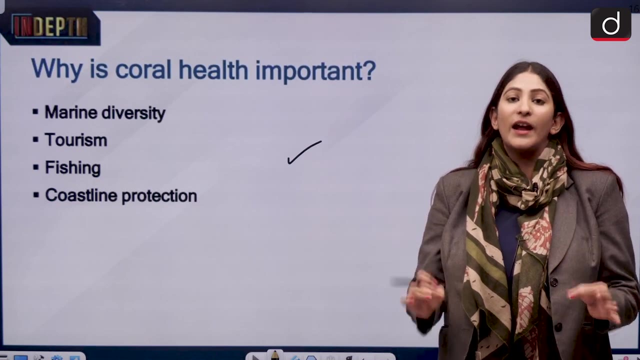 proper stock of fish, proper marine and aquatic animals, because many animals they thrive in corals. It is important that for shelter and food we maintain these corals, For tourism, such places which are thriving, which have a great thriving coral reef, atolls, fringing reefs. they get a 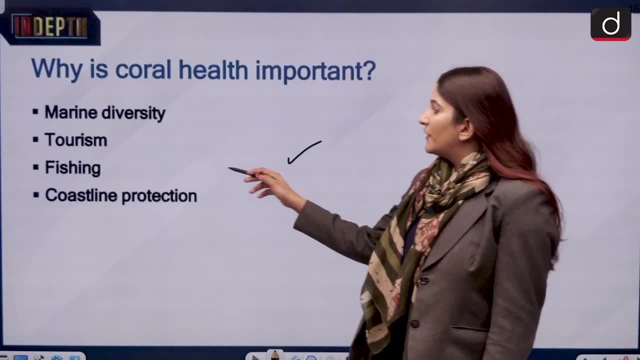 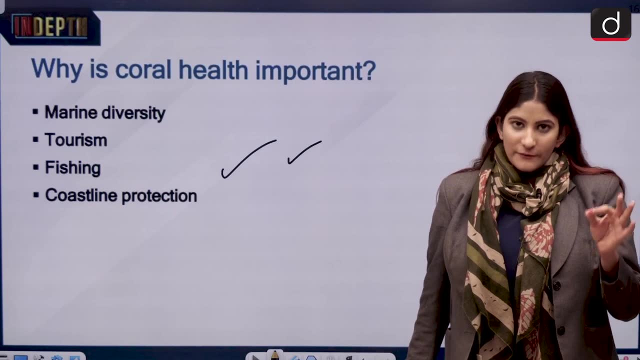 lot of tourists because they are very beautiful in nature. Then fishing For fishing. of course there are many fishes that are dependent on corals. If you remove the coral, then fishes will also not live there. That will take a toll on the livelihood of fishermen. Coastline protection. 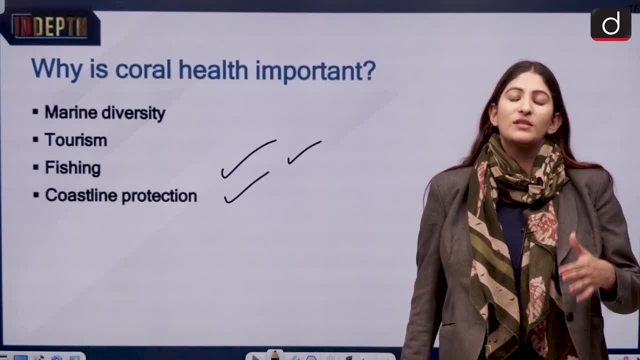 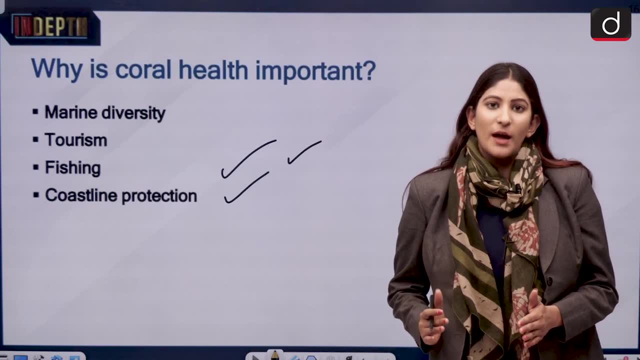 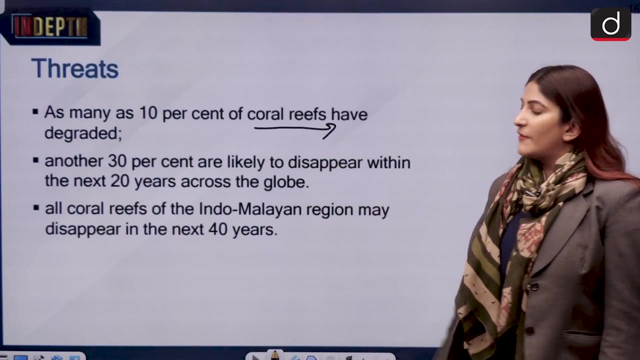 The Great Barrier Reef has protected Australia's coast from many issues, and these reefs are important to break the waves of tsunami, like mangroves, So for that also, it is important to maintain them. Now, as many as 10% of the coral reefs have degraded and another 30% are. 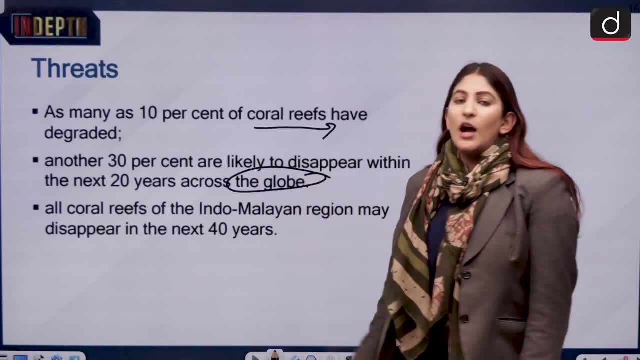 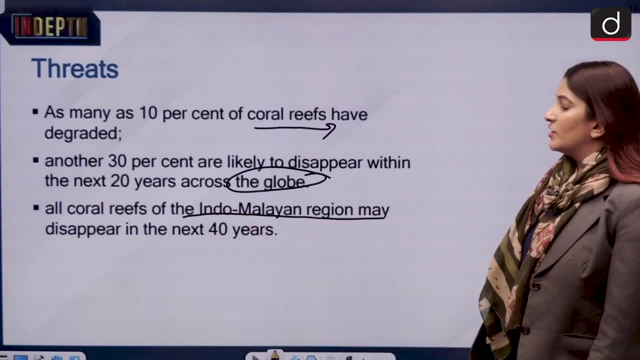 likely to disappear within the next 20 years across the globe. According to a study, if proper steps are not taken to conserve the coral reef- all coral reef of the Indo-Malayan region- they may disappear in the next 40 years. So it is important to first of all have an integrated 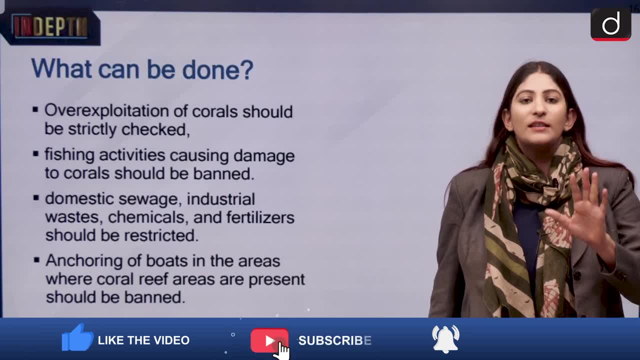 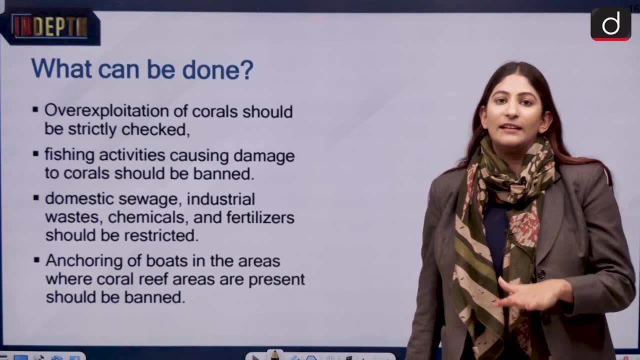 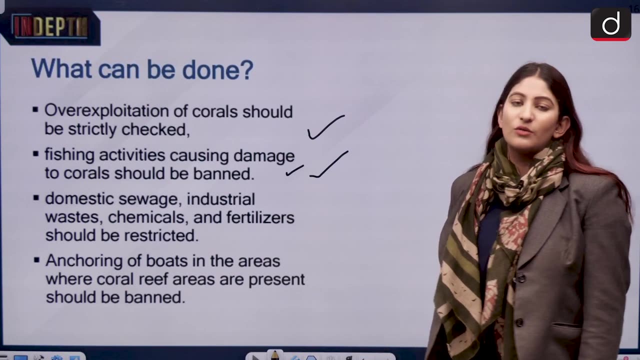 coral management plan that is not only for an area specific but also for world specific. You can have one policy and then delegate it. Overexploitation of corals should be strictly checked, Then fishing activities which cause damage to corals should also be checked. 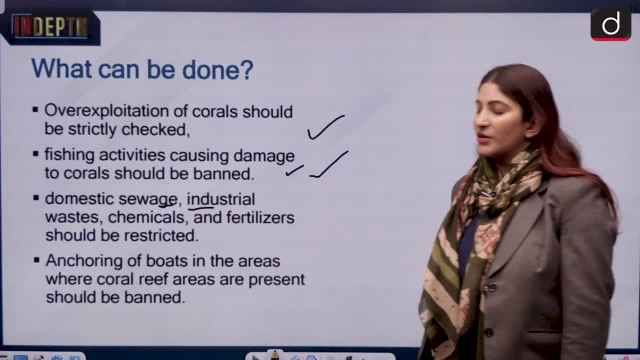 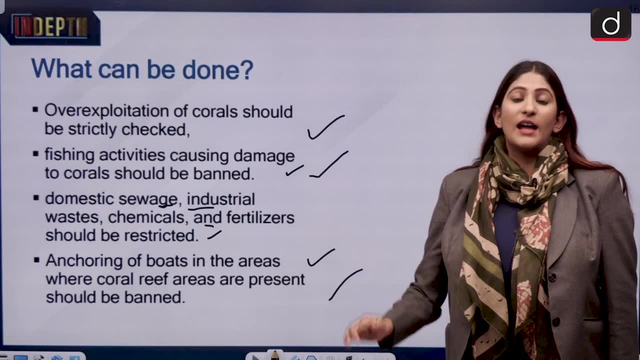 There should also be a checkup on domestic sewage, industrial waste, tourist waste, chemicals and fertilizers. anchoring of boats in the area where corals are present should also be checked, because these anchors can take out the corals all at once. So I hope. 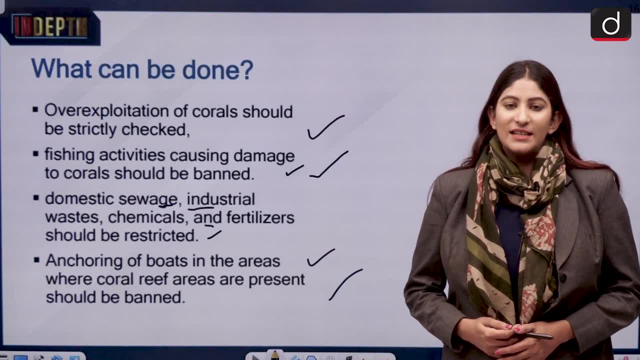 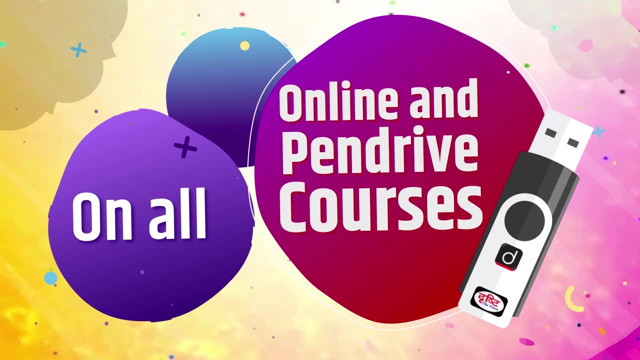 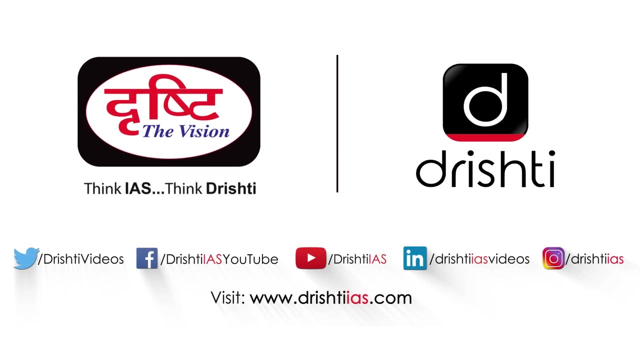 you understood all about coral reef. That's it. Thank you so much for watching. Transcription by ESO. Translation by —.